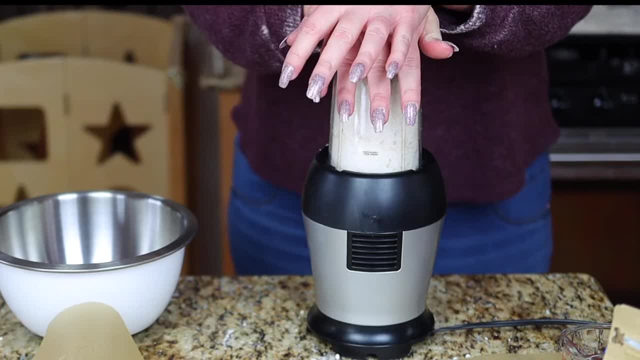 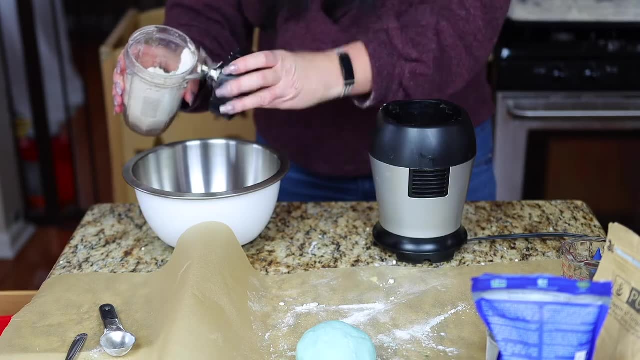 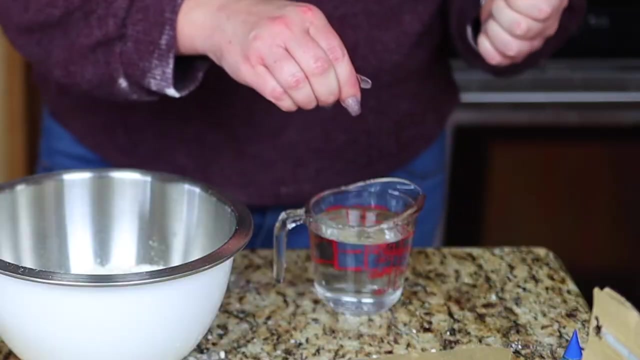 two cups of oatmeal and ground it up in my little nutriblender Once it had no more clumps in it. I then went ahead and dumped it into a large mixing bowl before adding one cup of flour. You're then going to take your flour and add it to the mixture. You're then going to take your flour. 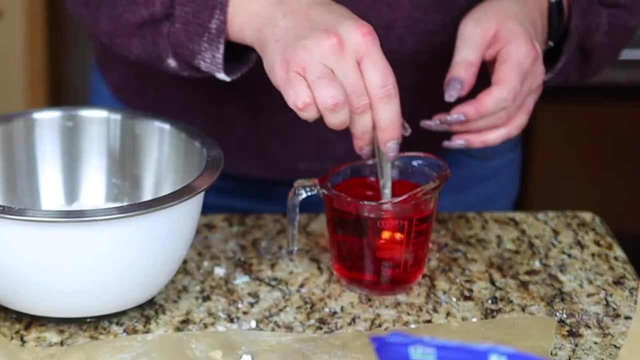 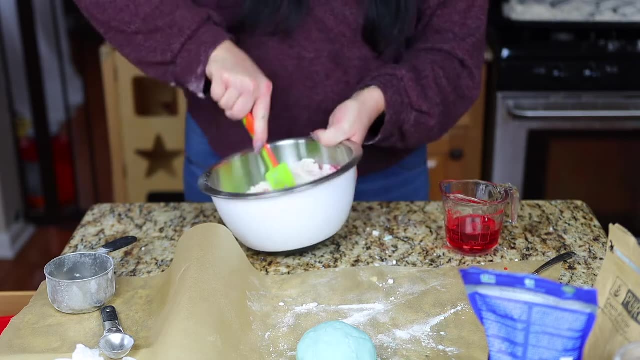 and then add a cup of warm water and then add as much food coloring as you'd like it to have and then stir it up and then again slowly mix it into your dry mix. I honestly felt like I added so much food coloring and it really still didn't come out like super. 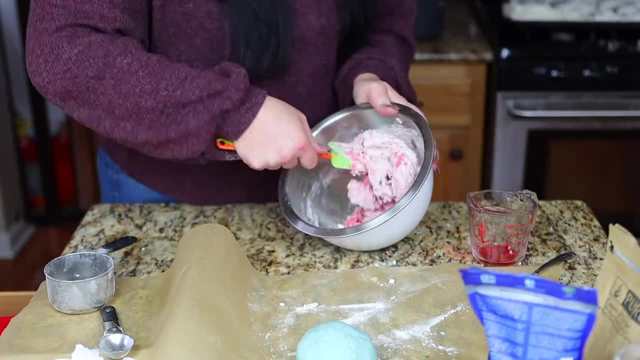 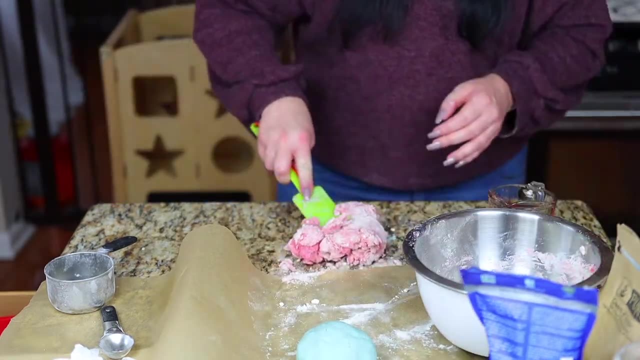 super pigmented, like I wanted it to. So feel free to as crazy as you want with that. You're then just going to stir it until it's all combined, just like we did with the first recipe, and then dump it out onto a table or whatever surface you're working on and continue to knead it. 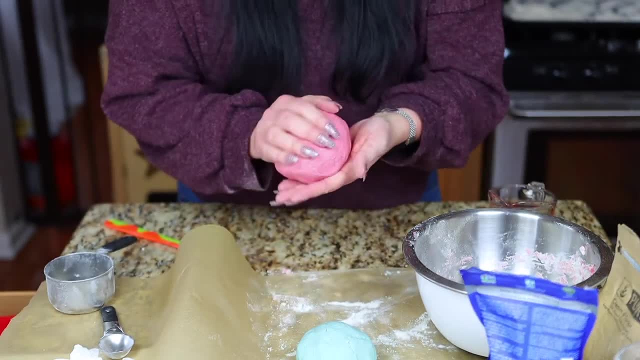 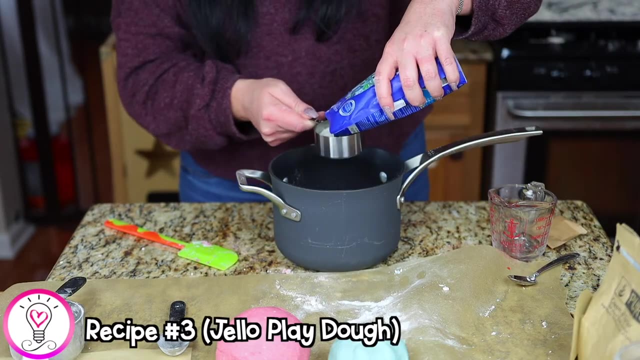 with a board. Here's how it looks whenилась it sounds like it won't have any biscuits in it. After your hands again until it's not sticky. our third recipe is my personal favorite, which is jello play-doh. so i make this right in a pot, because we are going to have to cook this on the stove. 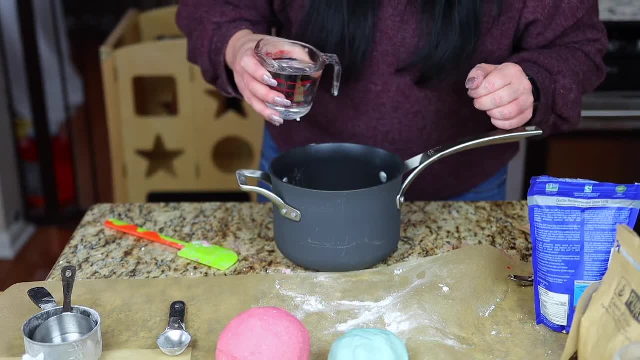 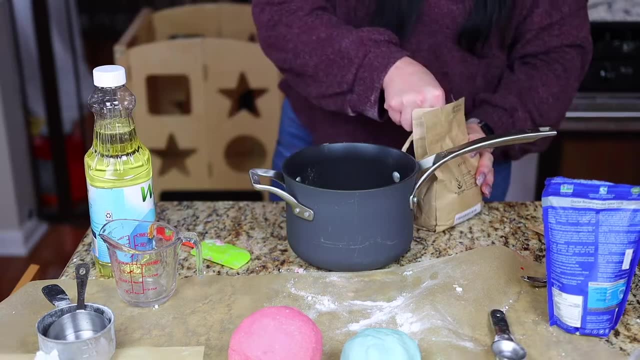 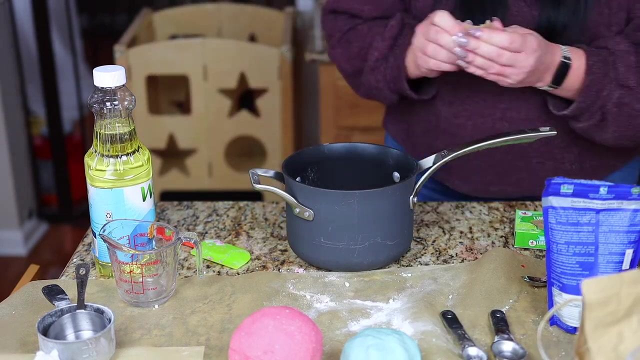 so you're just going to start with one cup of flour and then add half a cup of salt, and then one cup of water and one tablespoon of oil, two teaspoons of cream of tartar and then one package of unsweetened jello. i love using the unsweetened because it doesn't have the sugar. 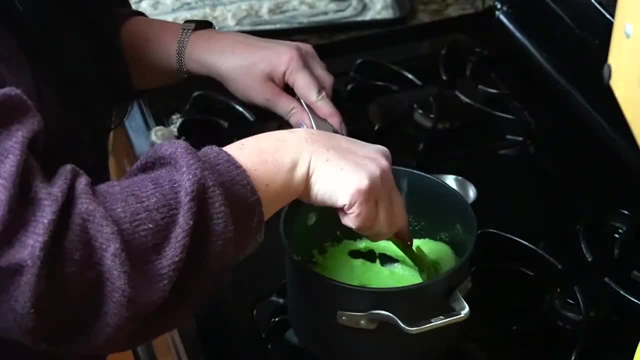 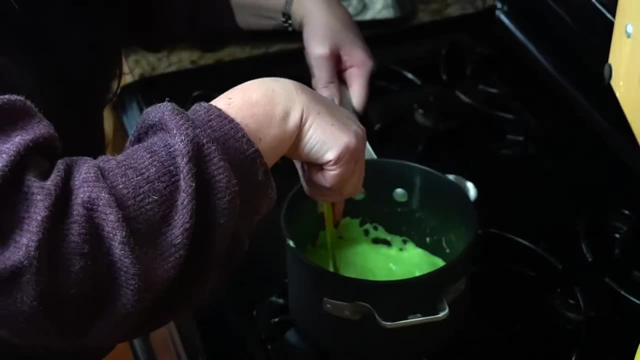 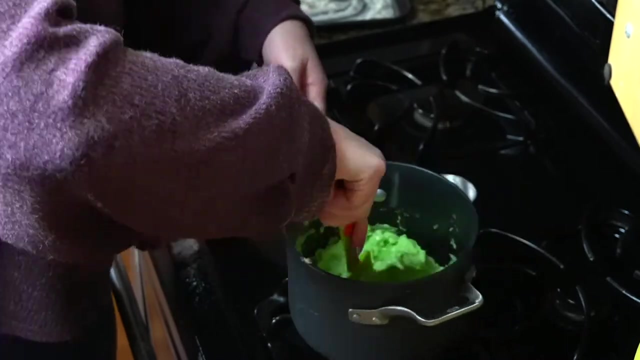 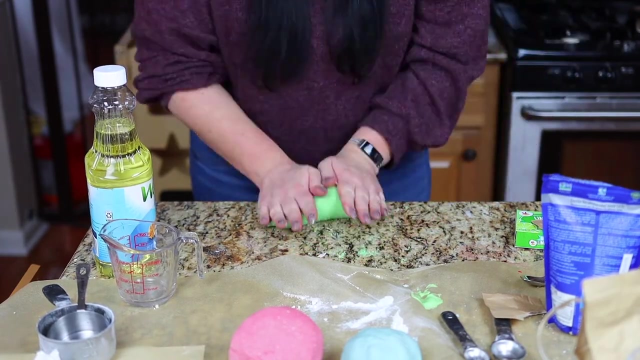 which makes it sticky. you're then going to mix all the ingredients together over medium heat on the stove and stir constantly until it starts to stick together. so you'll start to notice it'll get almost like mashed potato consistency. once it gets to that consistency you can take it out of the pot and then 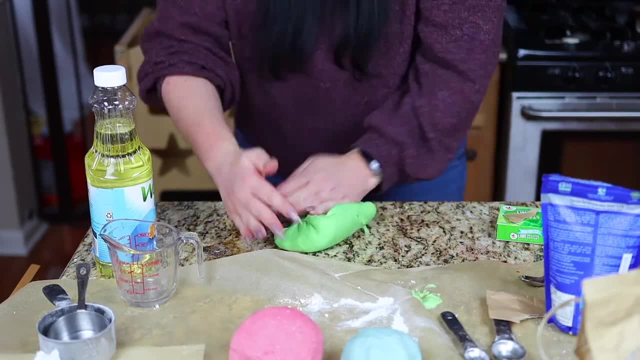 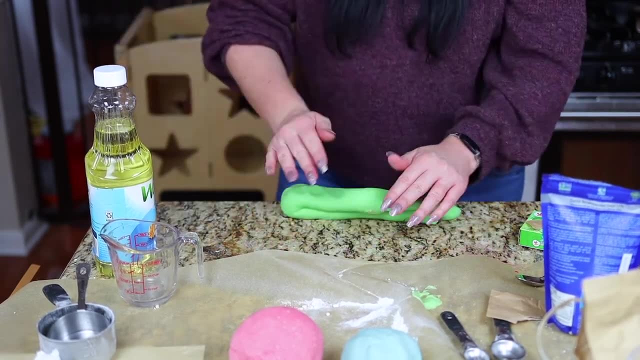 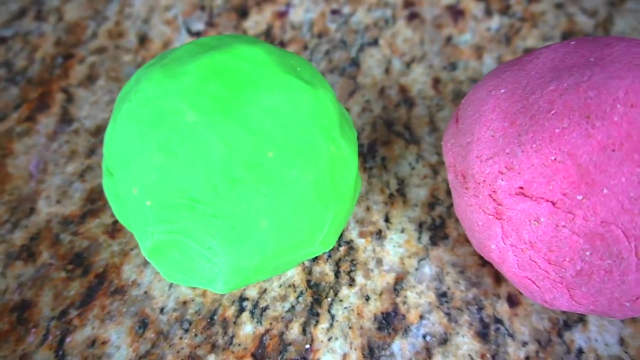 knead it on the table or whatever surface you're working on, Just be careful. obviously, if you're taking it right off the stove. it is going to be hot, so you should be still kneading it when it's warm, but just make sure it's cool enough for you to touch. There are our three taste: safe. 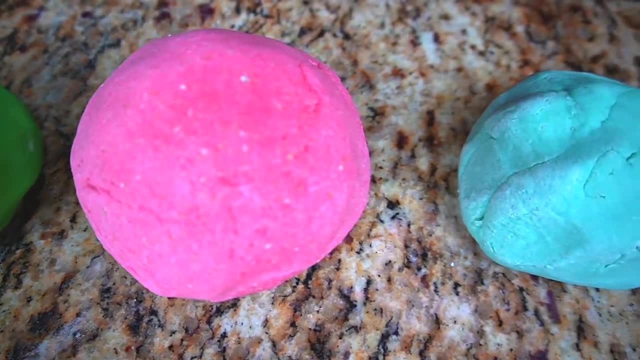 play-doh recipes. I hope you guys enjoyed this video. Please give it a thumbs up if you did, and don't forget to subscribe before you go. Thanks for watching.